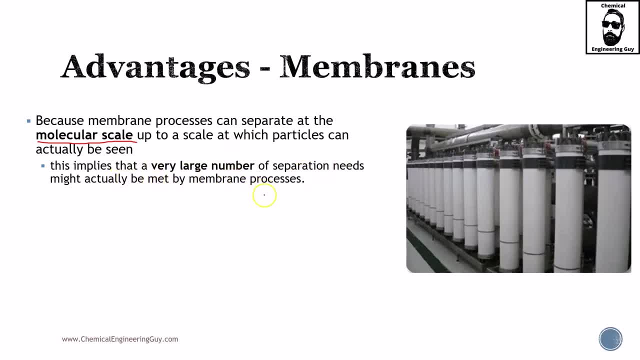 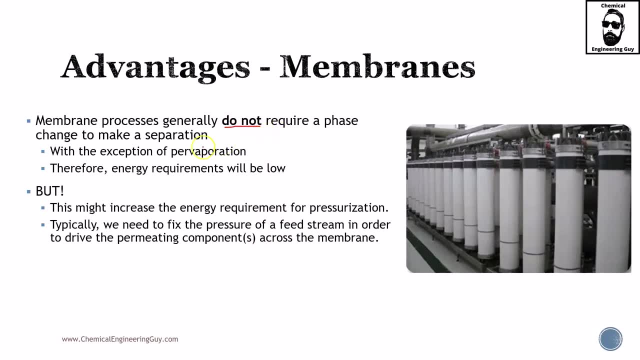 where is it? macromolecules, micromolecules, ions and so on. Membrane processes generally do not require a phase change, with the exception of pervaporation. but for now let's assume that we are not going to be changing overall the phase, And this is great because typically change on phases will. 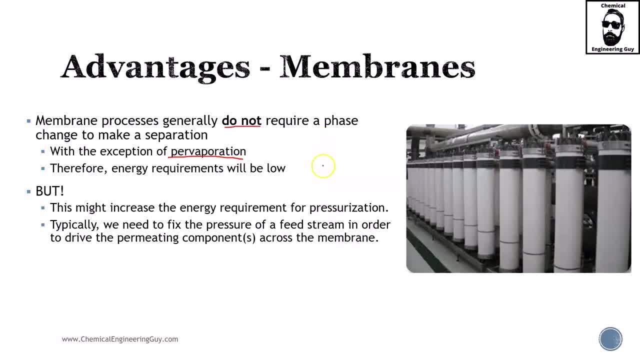 require a change on pervaporation. So let's look at the common advantages on membranes. So, for example, if you have a change on pressure or a drastic change on temperature which typically requires either work or heat, overall energy requirements which are expensive And the main. 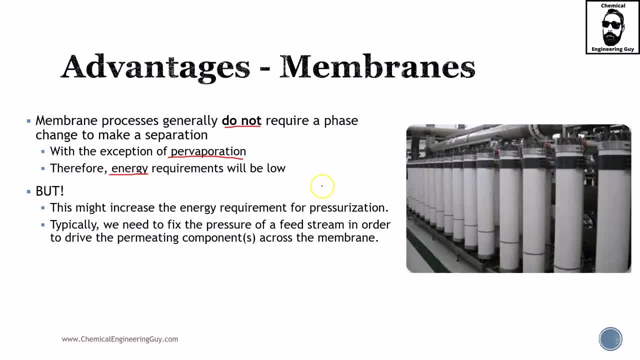 advantage to the membrane is that you do not require such changes on phase, But this might increase the energy requirement for pressurization. In some cases the change in pressure is even greater than the energy that we will require for heating or cooling. Typically, we need to. 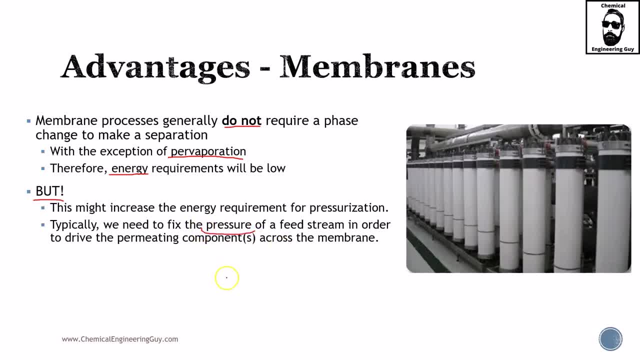 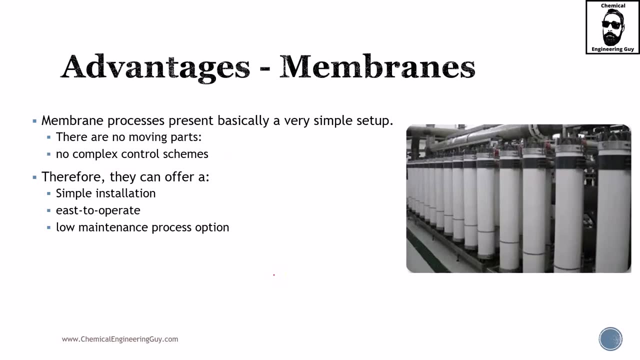 fix the pressure on the feed stream in order to drive the permeating components across the membrane. So we're going to encounter this a lot, especially when we are working with a membrane that we need to fix and set up the pressure in order to achieve the separation or achieve the permeation. 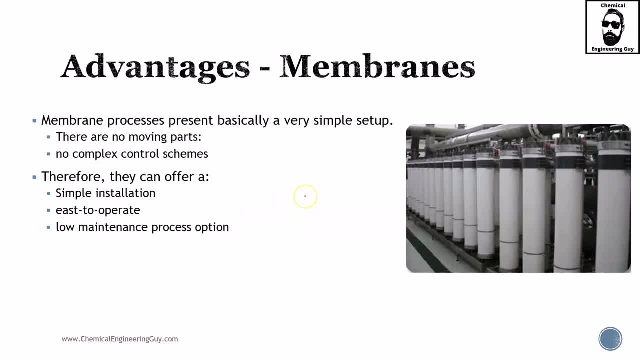 Membrane processes present, basically a very simple setup, So that's also a great advantage. I stated before, many of them come in cartridges, So once the equipment is installed, changing or the maintenance of the equipment is actually very easy There. 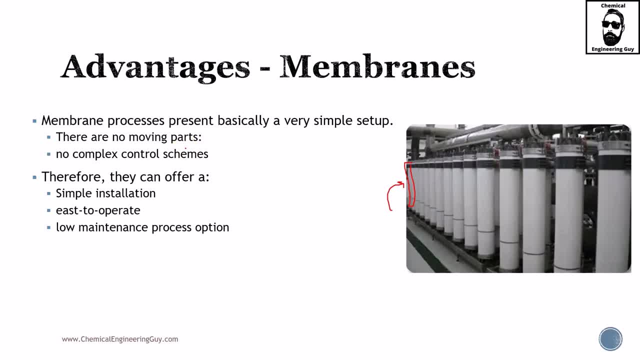 are no moving parts, such as in a condenser, re-boiler, compressor, and there are no complex control schemes. You are not going to encounter very complicated controlling systems. Therefore, they can offer a simple installation, easy to operate, which I think is one of the best. 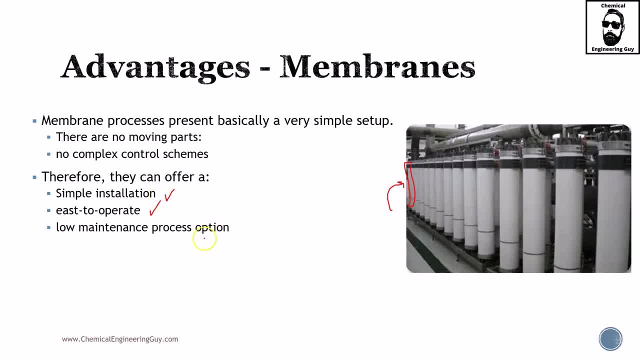 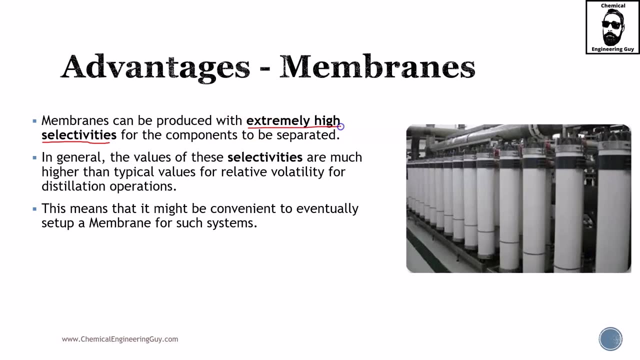 or easiest or more convenient aspects of membranes, and also the low maintenance process, which is either low in activity or low in, let's say, complexity. Membranes can be produced with extremely high selectivities. That's also a great advantage. Not only is it going to be cheap to 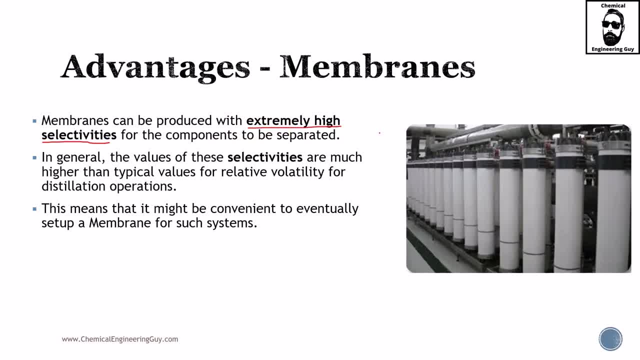 operate and install, but it's also very efficient for certain processes. In general, the values of these selectivities are much higher than those typically stated in conventional processes such as distillation. technically speaking, the volatility change, or maybe, in gas absorption, the solubility change on the gas, and so on, This means that it may be.